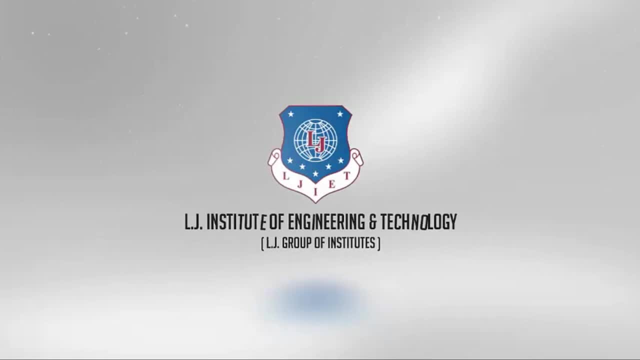 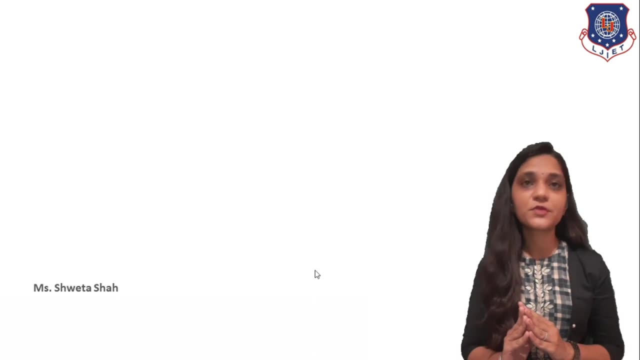 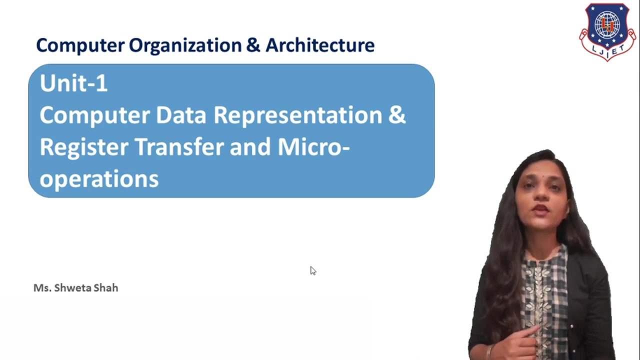 Hello everyone, my name is Shraddha Shah. We are here for the subject computer organization and architecture and in this subject we are going to start with unit 1, that is, computer data representation, register transfer and micro operation, and from this unit we are going to start with topic, that is, basic computer data types and component. 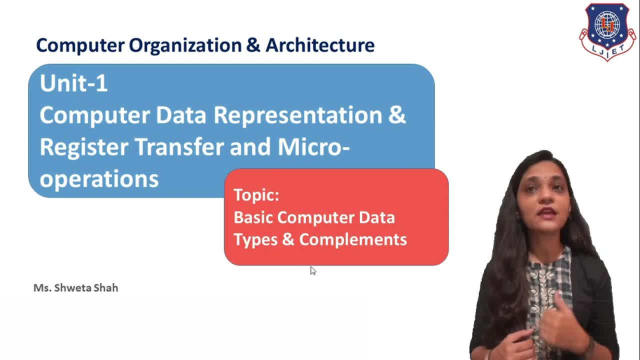 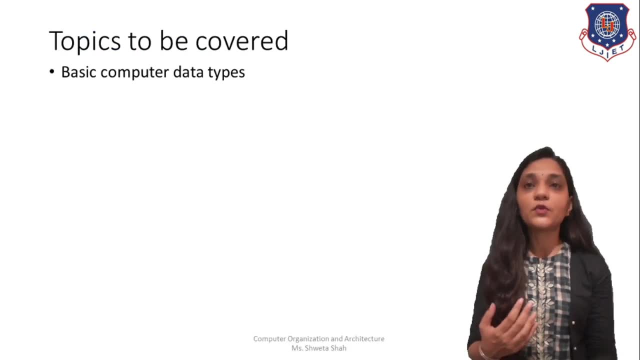 Before starting with this topic, let me see what are the outlines for this unit, What are the topics that we are going to cover in this unit? and these are basic computer data types and complements. Then we will see how you can represent your binary numbers in terms of fixed point representation and floating point representation. 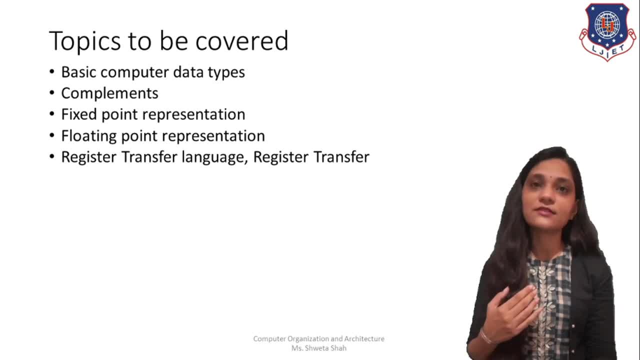 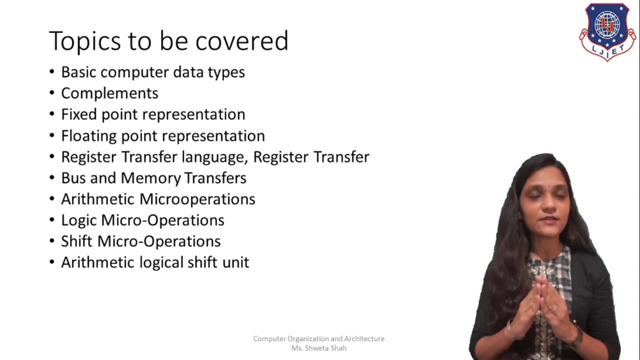 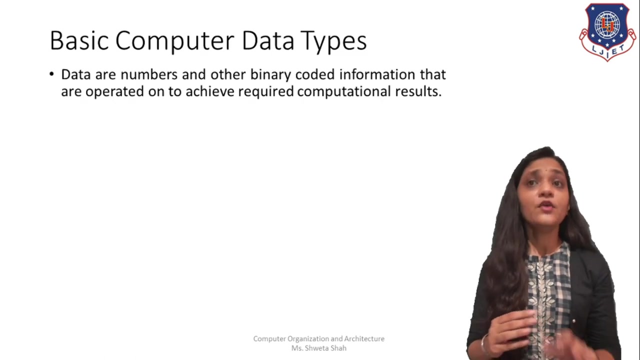 After that we will see register transfer, language and register transfer bus and memory transfer, and then we will see arithmetic operation and logical operation and shifting operation on binary numbers and lastly we will see arithmetic and logical shift unit. Okay, so let me start with the world topic, that is, basic computer data types. We all are aware that data are the numbers and other binary coded information that are operated on to achieve the required computational result. 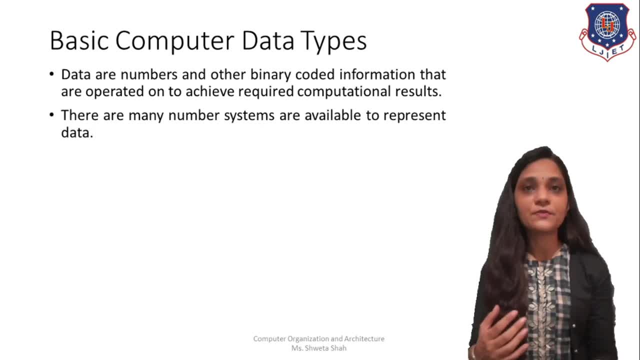 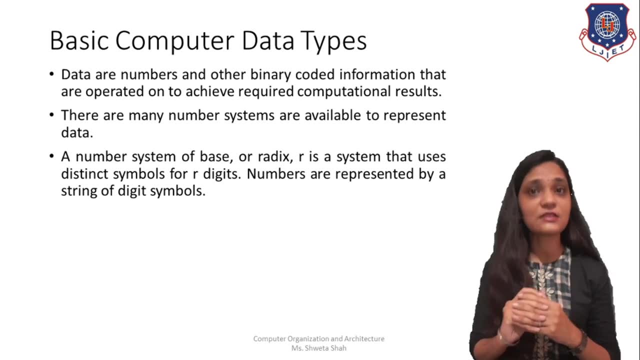 There are many number systems are available to represent the data. A number system is a system of numbers. A number system is a system of numbers. A number system is a system of values or radix. R is a system that uses distinct symbol for R digit. 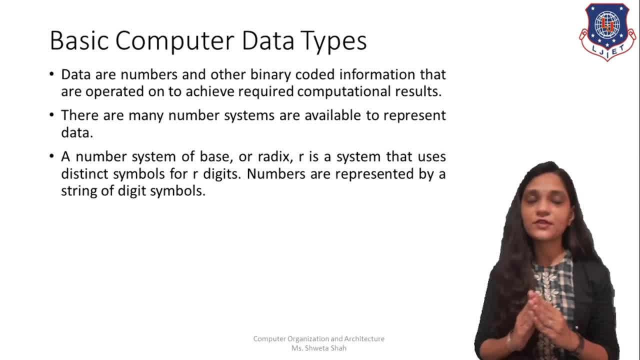 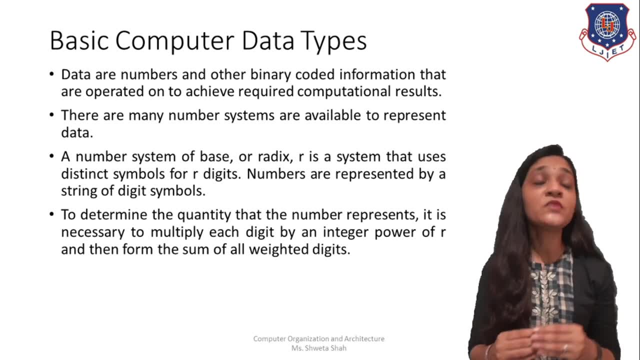 And the numbers are represented by a string of digital symbols, And to determine the quantity that this number is representing, it is necessary to multiply each digit by integer power of R and then form a sum of all weighted digits. Okay, so let me see with one example. 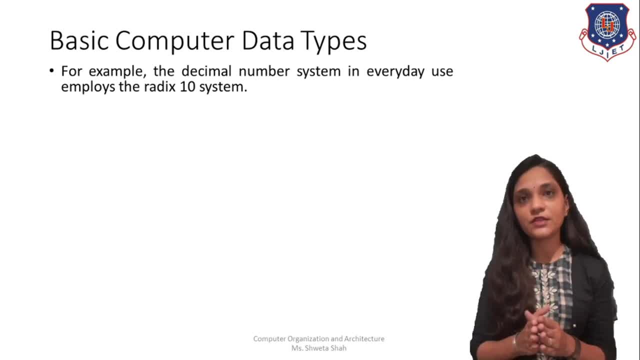 For example, if we have a decimal number system, decimal number system that we are using in every day, and that is radix 10, that means you can say waste 10 system and it is having total 10 symbols like 0, 1, 2, 3, 4, 5, 6, 7, 8, 9 and okay, uh, so we are. 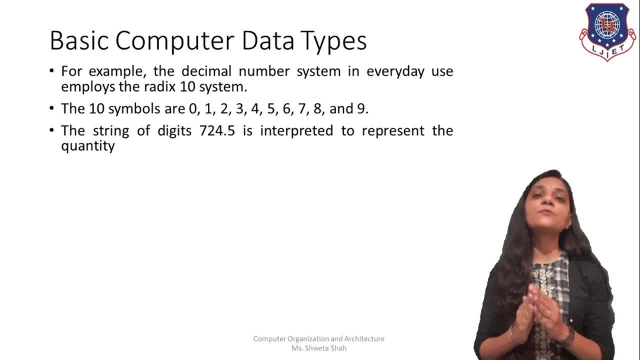 having here total 10 symbol and if we want to represent this string, that is 724.5, and we want to find out the what the quantity this uh string represents. okay, as we know this is, this is a decimal system, so the quantity will be same, but to represent this quantity we require uh multiply. 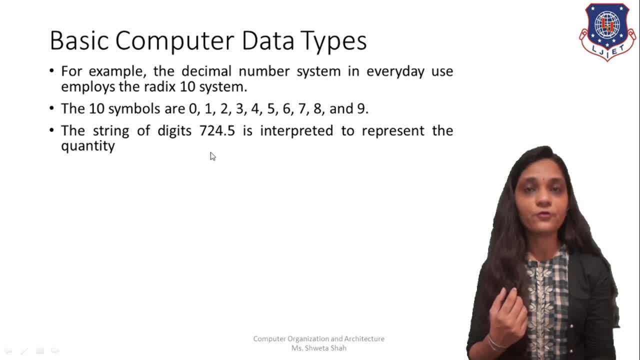 each and every digit, that is, 7, 2, 4 and 5, with, according to its position, power of 10. why power of 10? because this system is radix 10 and so it has a base 10.. so here for this string, we are going to represent the quantity, that is 7, 2, 4 and 5 with, according to its position, power of 10. why power of 10? because the system is radix 10 and so it has a base 10. so here for 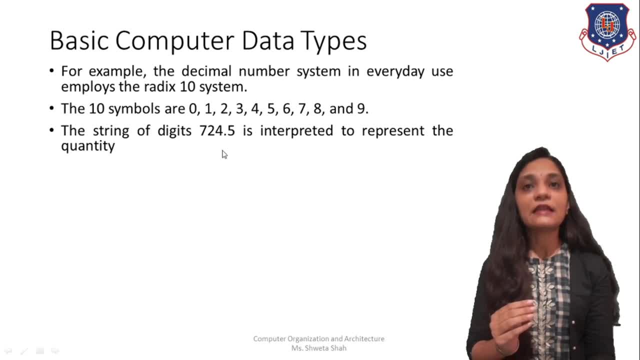 four is at zeroth position or you can say tenders to zero powers. position 2 is at tenders to one power position and seven is at tenders to 2, or you can say 100th position and similarly 5 is at tenders. 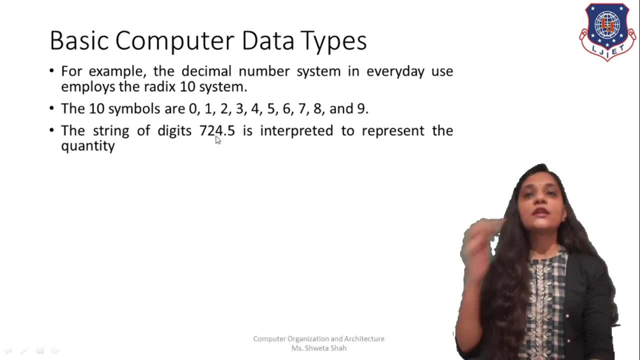 to minus one position. so to find out the quantity, we have to multiply this four with tenders to 0, this 2 with tenders to 1, the 7 with tenders to 2 and this 5 with tenders to minus 1, and we have to find. 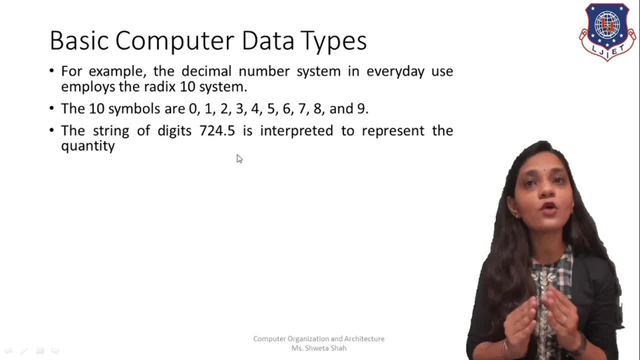 out the product. we have to find out the sum of this product. okay, this will be like this: 7 into 10 to 2 plus 2 into 10 to 1 plus 4 into 10 to 0 plus 5 into 10. 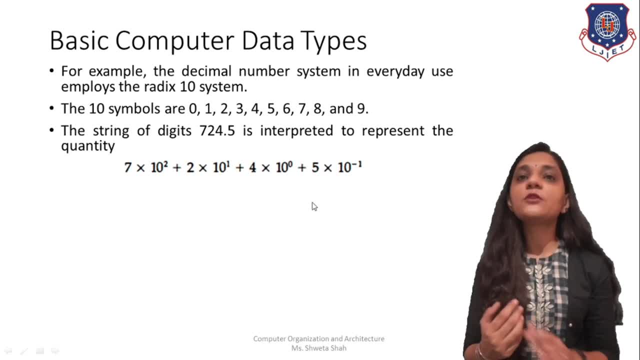 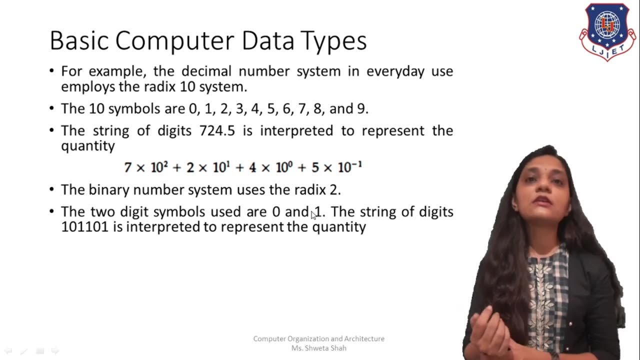 to minus 1. okay, so this quantity will be seven twenty four point five. but what if your number system is using relics to, or you can say, binary number system? okay, so let me consider one example. if we see that, if it system is a radix to system, 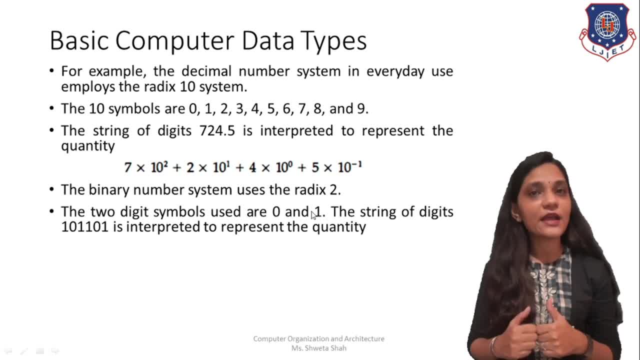 that means it has only two symbols that are zeros and one. okay. and if we have a string like this: one zero one, one zero one, and we want to find out if what quantity this string represents in terms of decimal. so what we require, we require to multiply in. 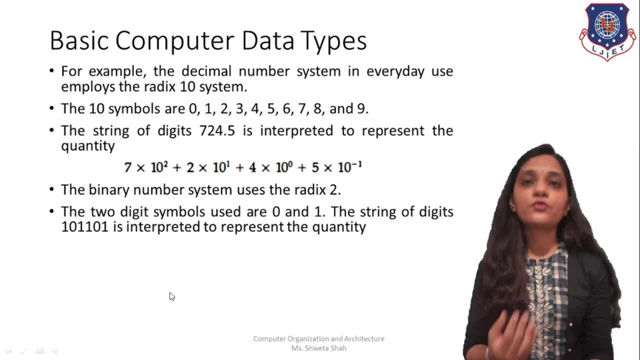 every ones and zeros with power of two according to its position. okay, so here: this one is at zeroth position, this zero is at one position, this one is at second position, this one is at third position, this zero is at fourth position and this one is at fifth position. okay, so. 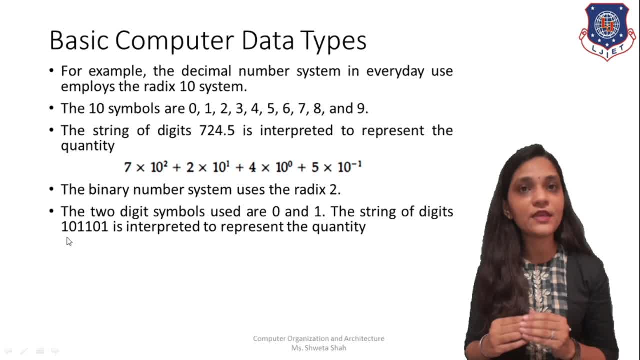 here we have used a radix two system. that means our base will be two. so we have to multiply each and every ones and zero with power of two, according to position. so it will be like this: this one multiplied by 2 is to 0. this 0 multiplied by 2 is to 1. this 1 multiplied by 2 is to 2. this 1. 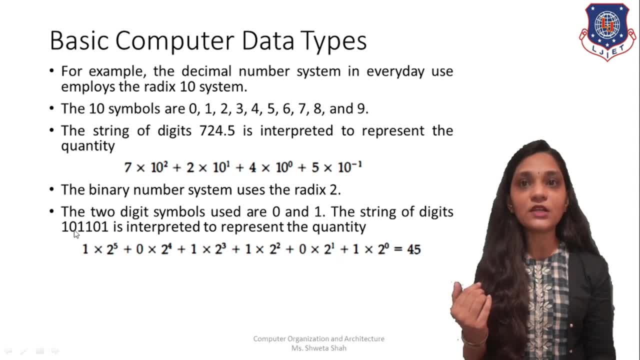 multiplied by 2 is to 3, this mark and the 0 multiplied by 2 is to 4, and this 1 multiplied by 2 is to 5, and if you equate this quantity, or you do, you can add this all partial product, then you will get the quantity. 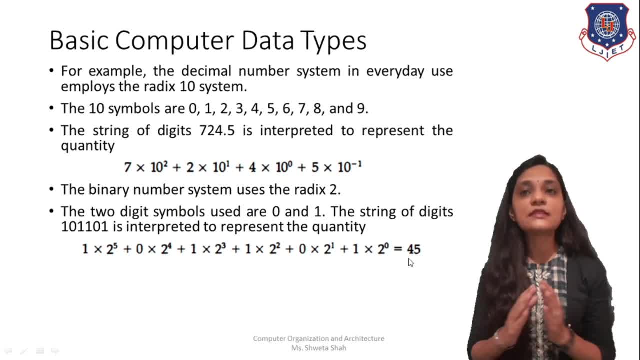 that is 45. okay, that means this string 1 0 1. 1 0 1 represents the decimal quantity 45. if you want to represent 45 in terms of decimal, you can write like 4 and 5. and if you want to represent this: 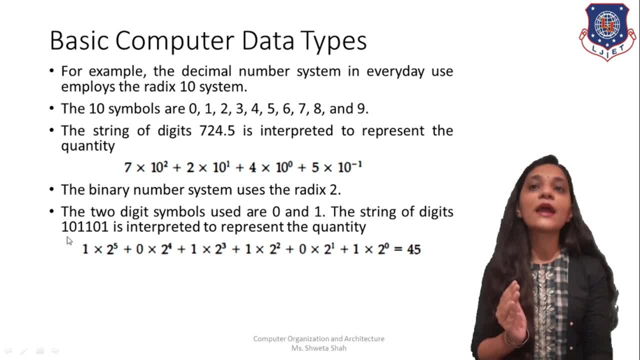 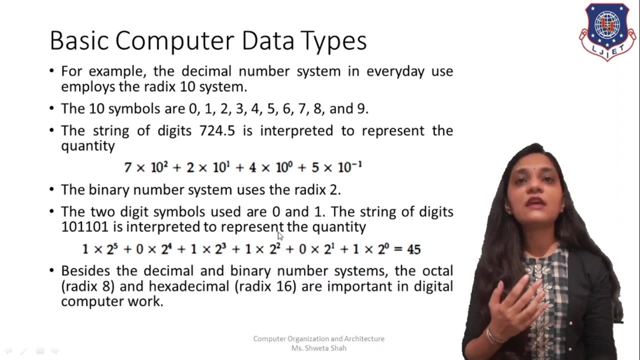 quantity in terms of binary, then you have to write like: 1 zero one, one zero one. okay, quantity will be same but representation will depend upon your number system, which number system you have used. okay, uh, this decimal and binary are not only two number system that you can use. there are so many number of systems like you can use: octal, hexadecimal, bcd. 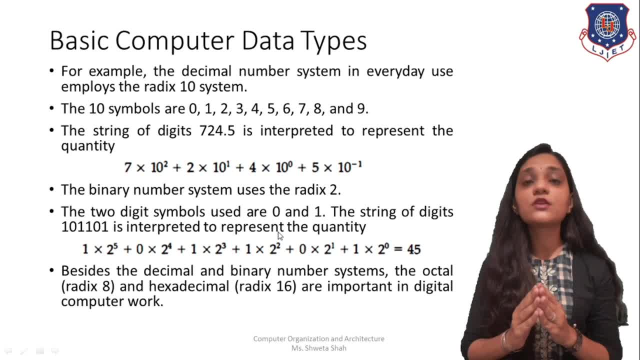 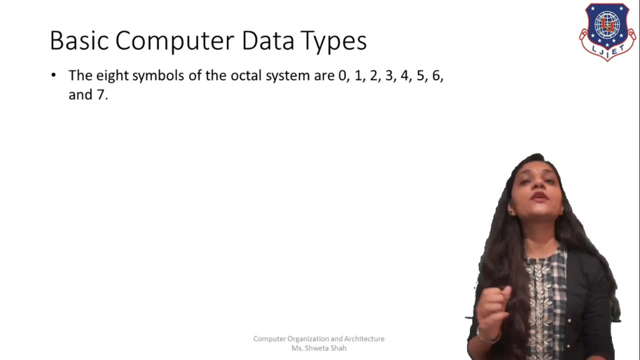 and so on. okay, uh, for example, you you are using octal number system, then it is already eight number system. hexadecimal number system is a radix 16 number system. that means it has a total 16 symbols. okay, how the system source works. let me see, for example, if we consider the octal number, 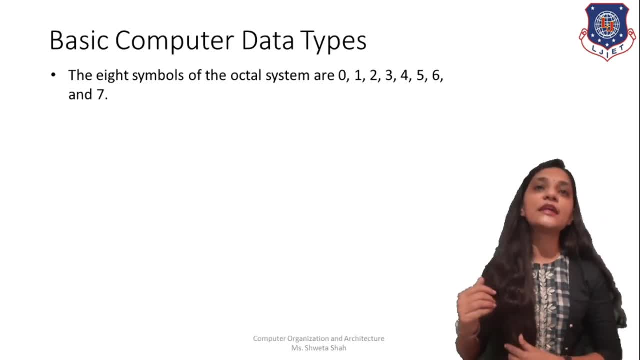 system, that is radix eight system, and it has a total eight symbols like zero, one, two, three, four, five, six, seven. okay, and for any number system, whenever you are going to use this with the digital system, you have to use the binary conversion of that number. okay, so for this, 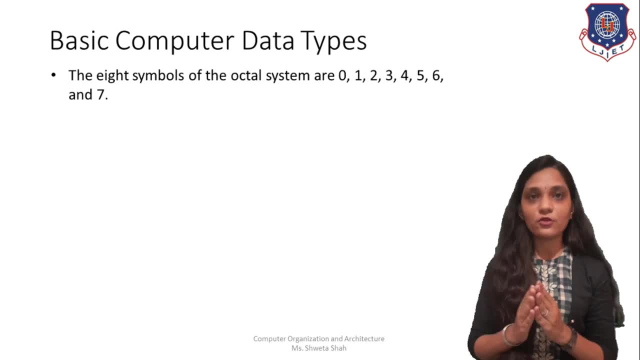 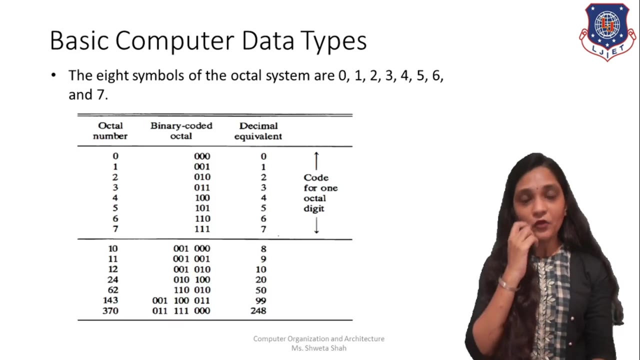 octal representation, we have total eight symbols, and to represent eight symbols in terms of binary, with different, different bit pattern, you will minimum require eight patterns. okay, so for this we have this kind of eight pattern for zero. we are going to using zero, zero, zero for one, we are. 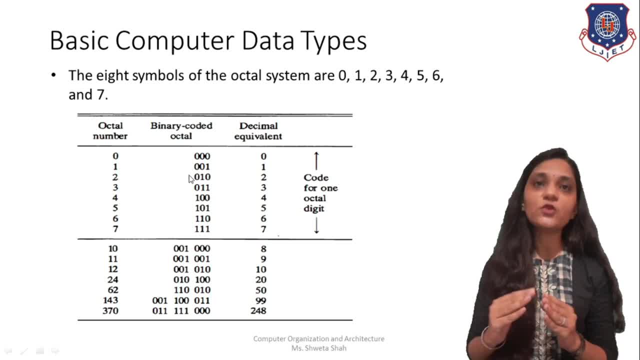 going to using zero, zero, one, four, two zero, one zero and so on up to seven. we have one, one, one, okay. and if you have a string of this octal number like 10, 11, 12, 1, 143, kind of that, so at that time you have to consider. 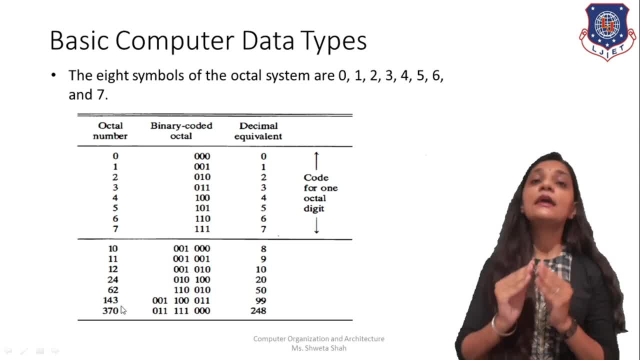 each and every octal number as an individual octal number and convert that number into binary. for example, if we consider number 62, so we have to consider this 6 as an individual binary, number 2 as an individual binary. let me consider string 62. okay, so for this 62 string, you have to. 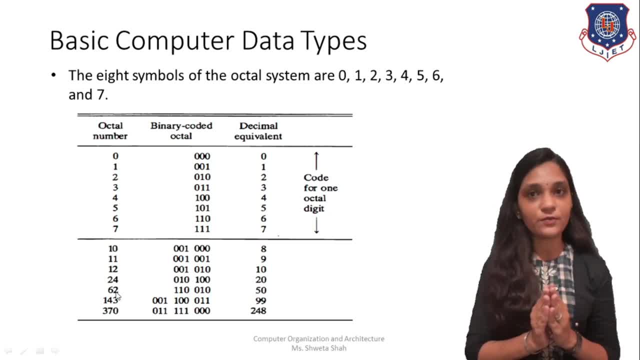 consider 6 as a different octal number and 2 as a different octal number. okay, so for 6, we have binary pattern as a 110 and for 2 we have binary pattern 0, 1- 0. okay, so by this way, by using this, 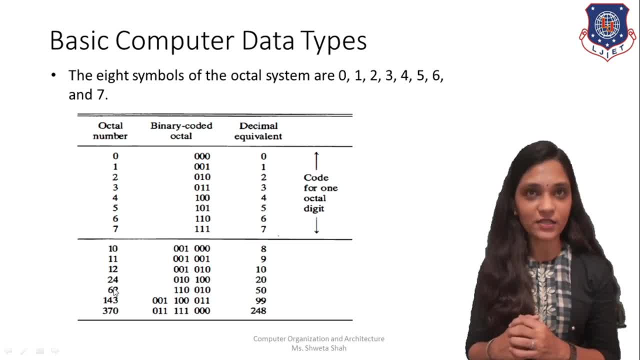 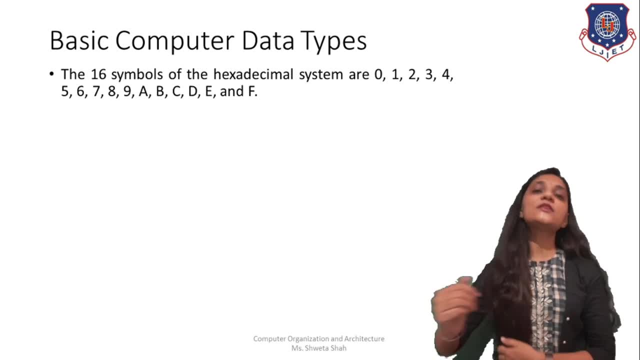 6-bit representation. you can uh represent this: 60 to 20 and soon, okay, uh. next let me see what is for hexadecimal number system. hexadecimal number system is a radic 16 or you system, so it has a total 16 symbols to represent this number system and their. 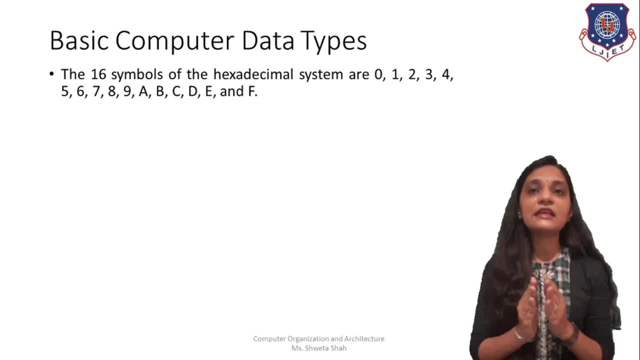 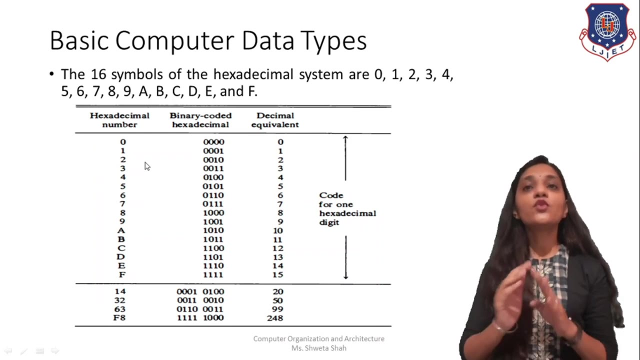 symbols are 0, 1, 2 up to 9, and then a, B, C, D, E and F. you have total 16 symbols, and whenever you considering this with the digital system, you have to convert this into binary system, and so for that conversion, you will have total 4-bit. 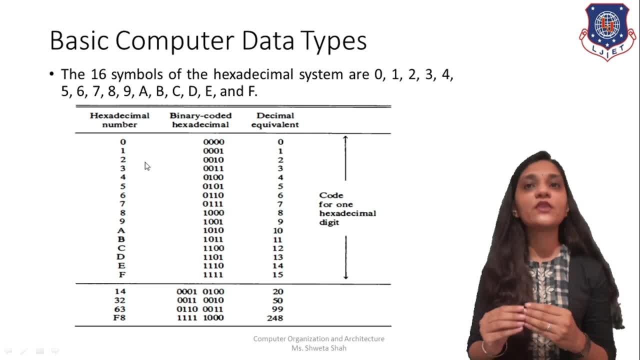 representation for each and every symbols. as you, we have total 16 symbols and we can represent the 16 symbol by using 4-bit binary pattern. so for 0, we have 0 0, 0, for 1 we have 0 0 0, 1, and for 2 we have 0 0 1, 0, and so on up to 9. for 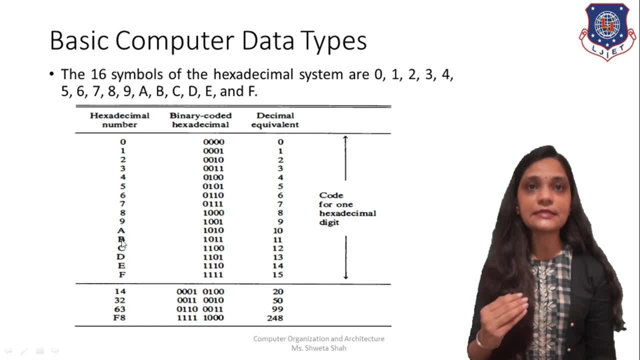 after that we will. you, we are going to using ABC symbols. ok, so for a, we have 1 0, 1, 1, and so on. and for F we have 1 1, 1, 1. ok, so all patterns you can perform by using 4-bit representation. we have used and we have assigned to each. 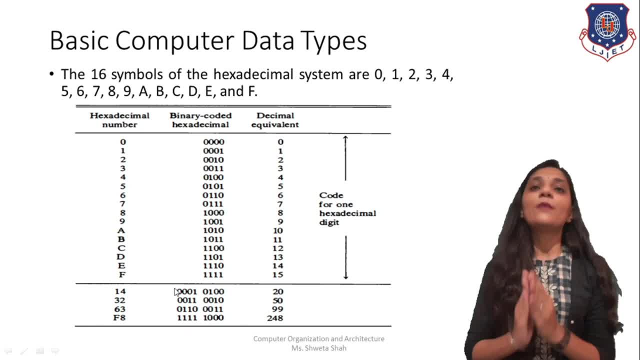 and every hexadecimal symbol. ok, so by this way you can use hexadecimal number system. if you have string of hexadecimal numbers like F, 8, 63, 32, so at that time, similar to octal number system, you have to consider each and every hex number as an individual number and convert that number into binary. so, for example, for 63, 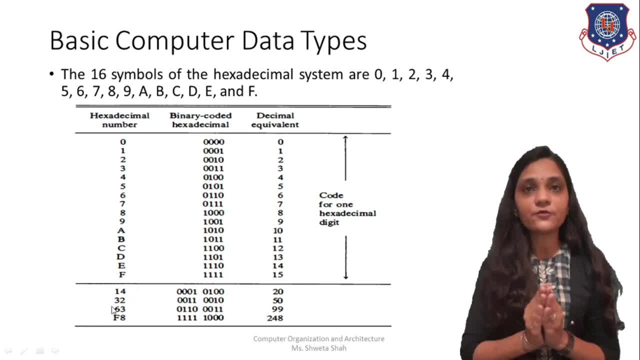 you have to consider 6 as a different hex number, 3 as a different hex number and convert 6 into its equivalent binary and 3 into equivalent binary. so you will have 4- 6 as 0, 1, 1, 0 and 4- 3 as 0, 0, 1, 1. ok, so by this way you can convert any. 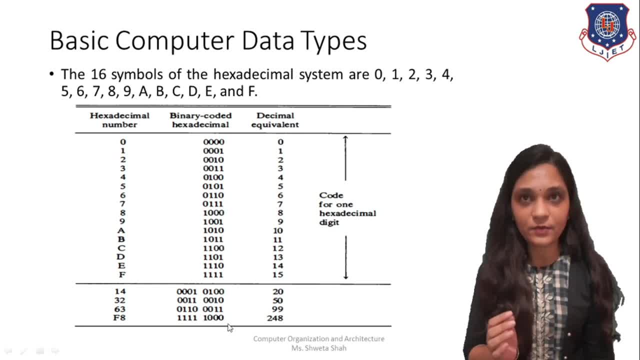 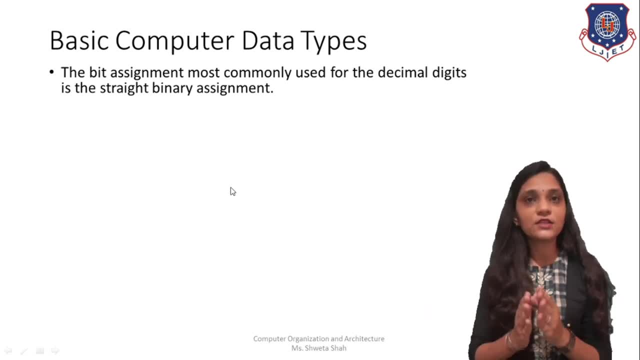 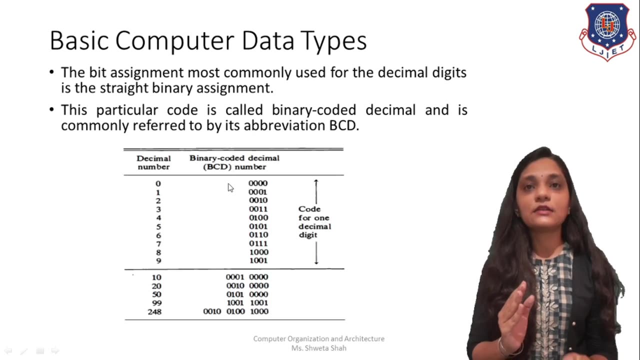 hexadecimal numbers into its equivalent binary number. one another system that we are going to use is a decimal number system that we are generally using. ok, in this system, we have total 10 symbols, ok, and that is 0, 1, 2, 3, up to 9. 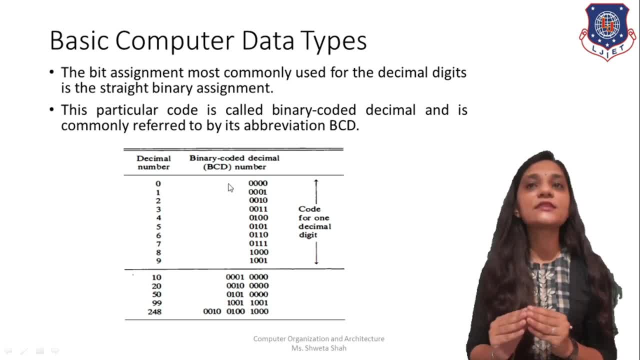 ok, only numbers and it is also known as a binary coded decimal, that is BCD. ok, and we have. if we have a string of BCD numbers, then we have to consider individual numbers and then convert it into its equivalent BCD code. ok, for 99, we have 1 0 0, 1 and 1 0 0, 1 individual 9 names. ok, so by this way we. 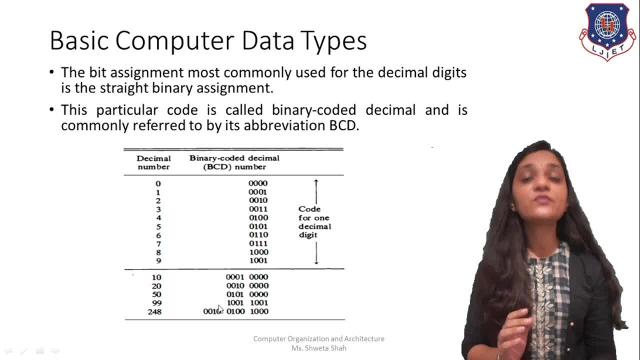 can consider a BCD number system. ok. so you can use any number system whatever you require, but ultimately you have to convert it into its equivalent binary and that will depends upon your number system, how you have designed your code. ok. so next we are going to see with the 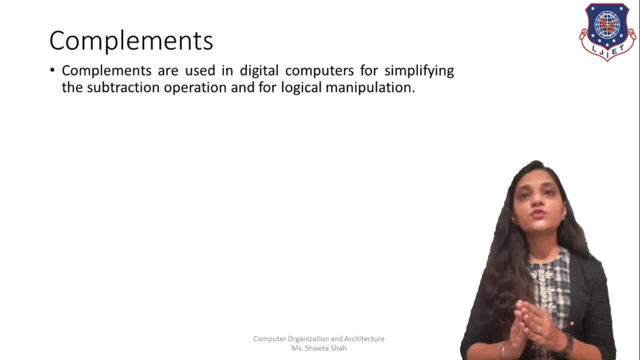 components. so the complements we are using in digital computers are generally for the simplification of subtraction operation, and you can also use this for logical manipulation, as we are aware that there is no circuit that you can design like subtract. ok, you can do subtraction operation, but by means of. 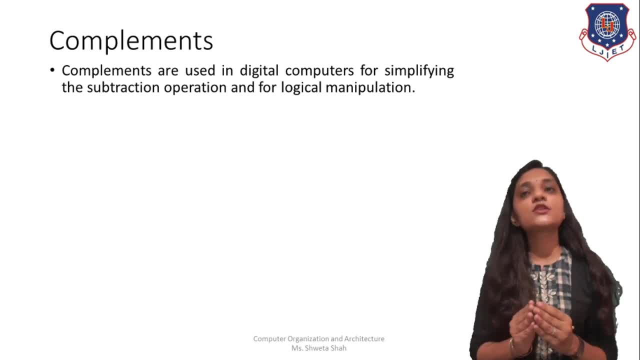 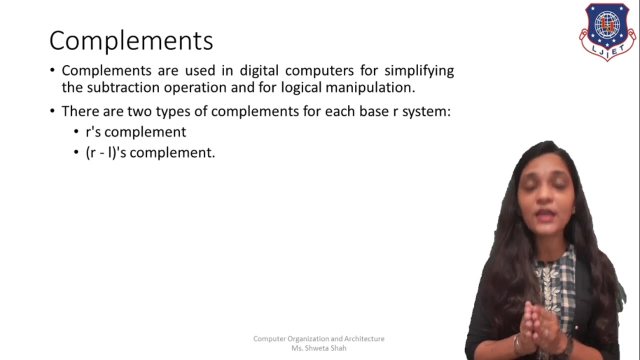 addition: ok, and for this addition you will require the complement of subtracted ok. and this complement can be two types, like as complement and r-1 complement. for base R system: ok. and for different, different representation of R you will have different, different complement. but each and every system will have two complements. for example, if you consider 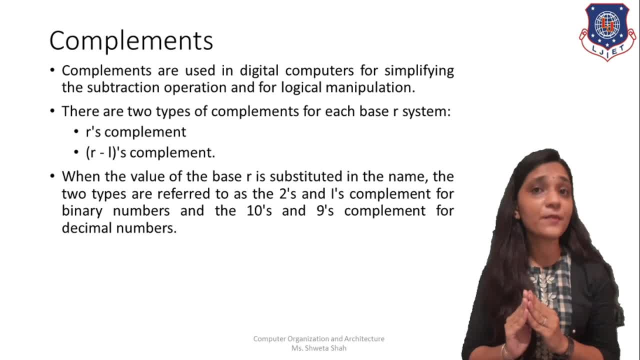 binary number system. that means it will have ways 2, that is 2. okay. so it will have two complements, like 2's complement, and 2 minus 1, that is 1's complement. okay, if we consider decimal number system, that is base 10 system. so it will have r's complement. 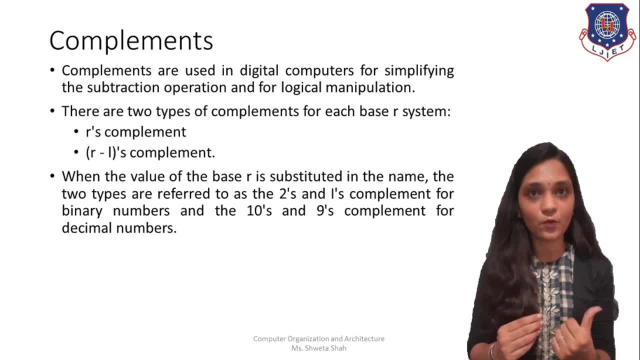 that is 10's complement and 10 minus 1, that is 9's complement. okay, and similarly for hexadecimal and octal number system. for octal number system you will have 8 complement and 7's complement, and for hexadecimal number system you will have 16th complement and 15th complement. okay, so, 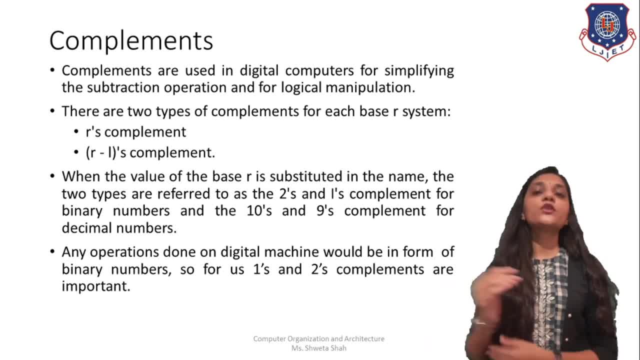 for us. we are, as we are going to, using digital machine and that are always going to work on binary numbers, and we are designing hardware in this course, so we will require generally 1's complement and 2's complement. okay, so let me see how you can design 1's complement and. 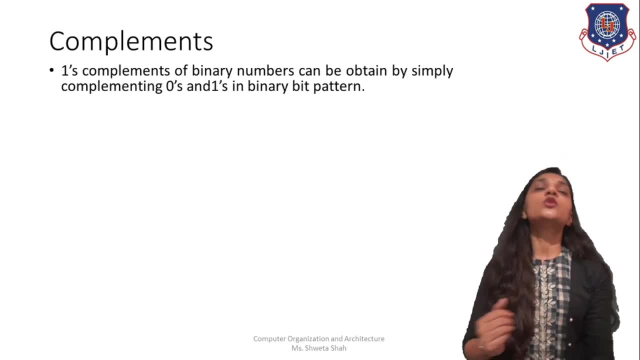 2's complement of the binary numbers. okay, so for 1's complement, you just require to interchange zeros and one in your binary string. if you are given a binary string and you are told to convert this into its 1's complement. so you just require to interchange 1's and zeros, okay, and for 2's complement you have to add one.